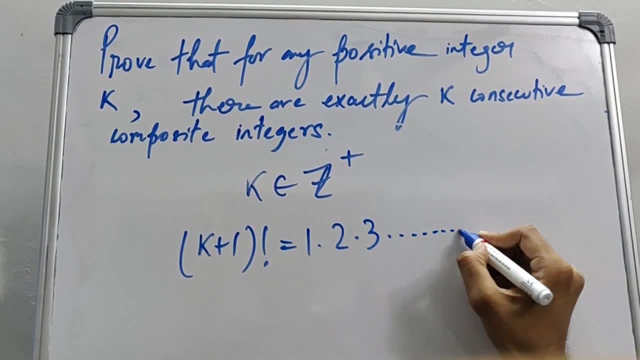 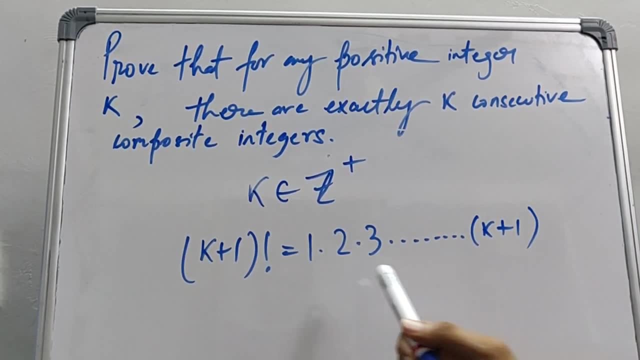 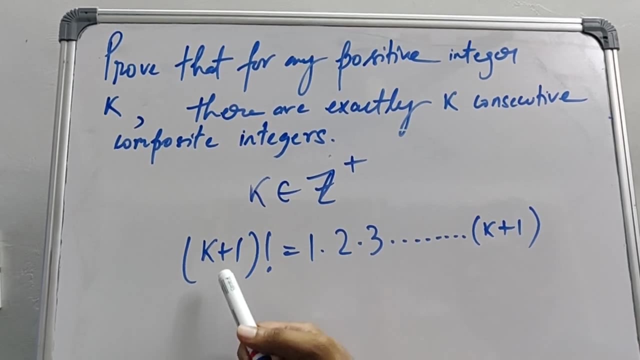 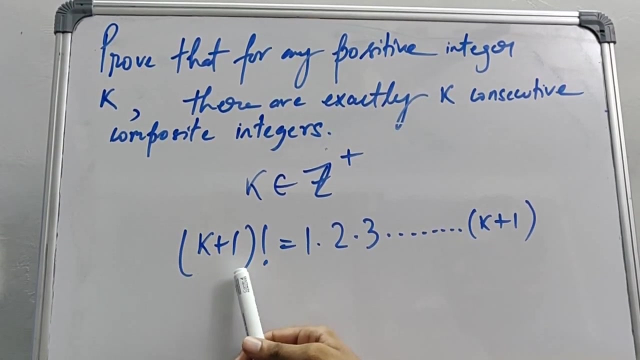 equals to 1 into 2, into 3, till k plus 1.. So from here it is easy to see that each of the term in this product is a factor of k plus 1 factorial. One is obviously a factor of any integer. Therefore one is a factor of k plus 1 factorial, And two is also a factor of k plus 1 factorial, and so on. So we can say that 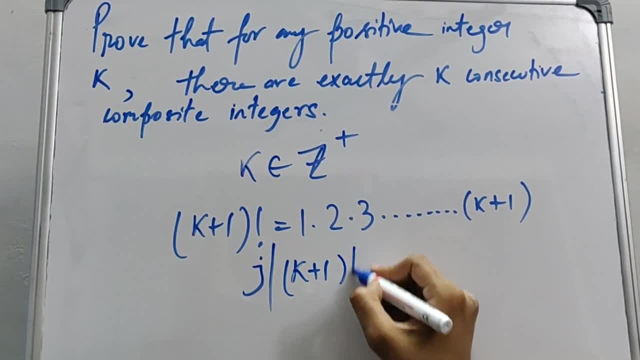 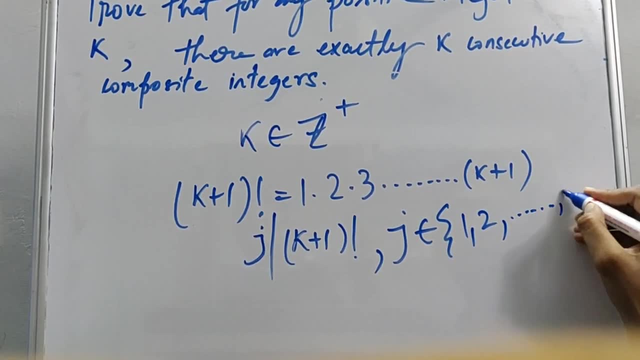 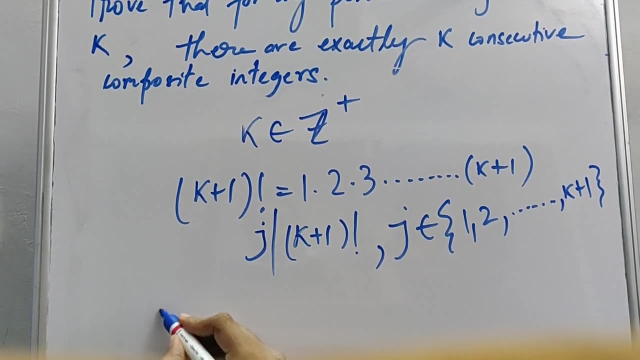 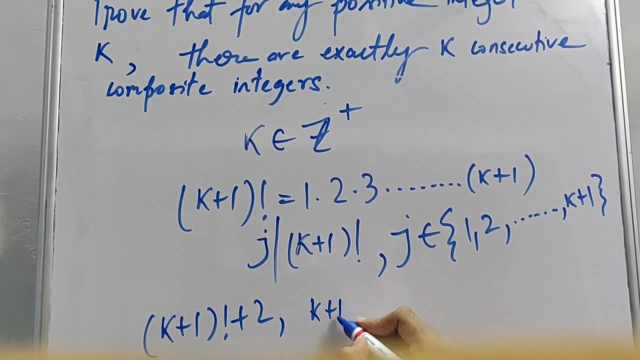 j divides k plus 1 factorial, where j belongs to the set 1 comma, 2 comma, dot, dot, dot k plus 1.. Now consider the integers k plus 1 factorial plus 2. Then k plus 1 factorial plus 3.. 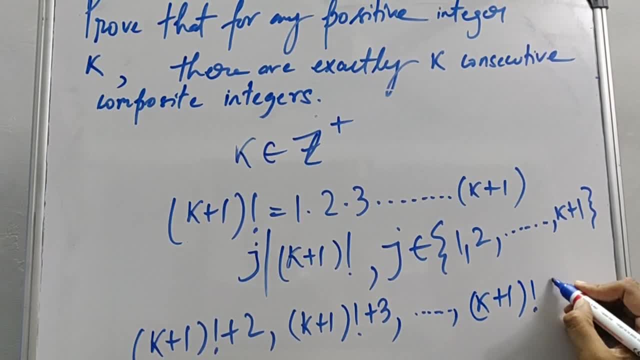 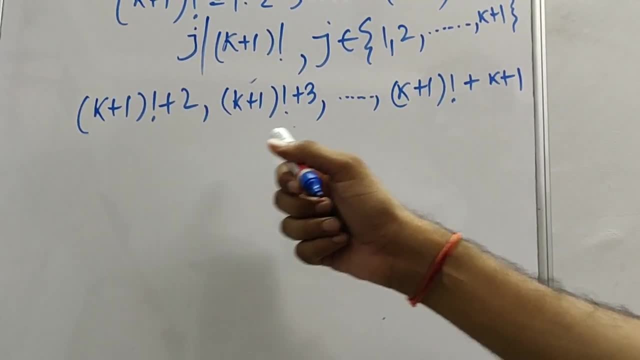 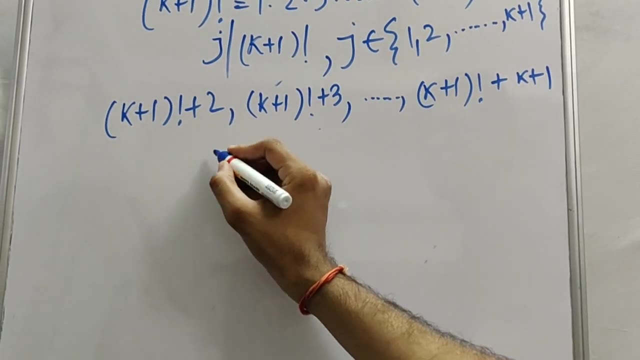 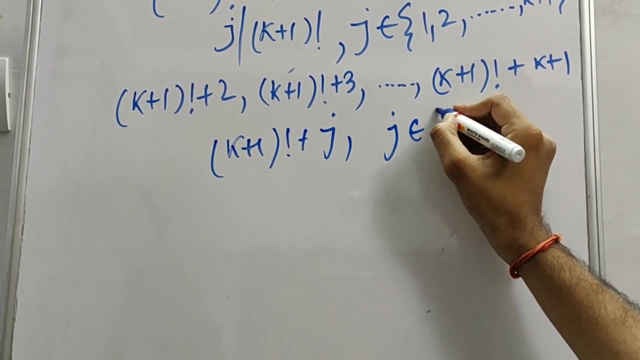 and the last one to be k plus 1, factorial plus k plus 1.. So we have constructed a sequence of k consecutive integers. We will show that each of them is composite. Now a general term of this sequence is of the form k plus 1, factorial plus j, where j belongs to the set 2 comma 3. 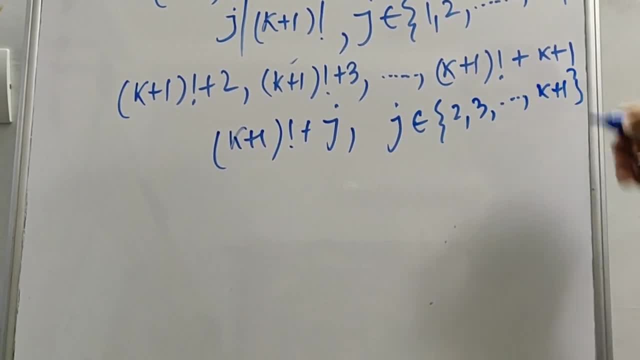 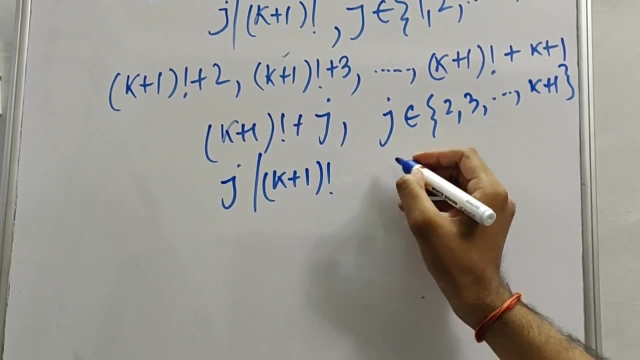 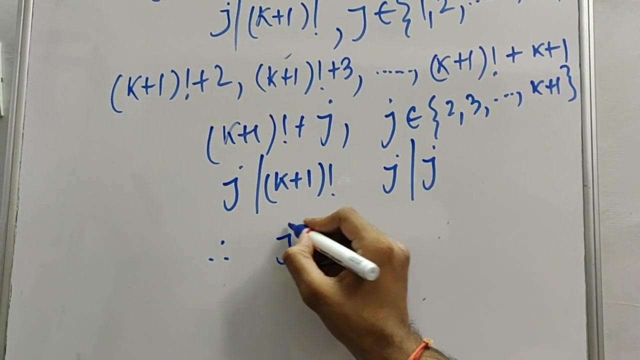 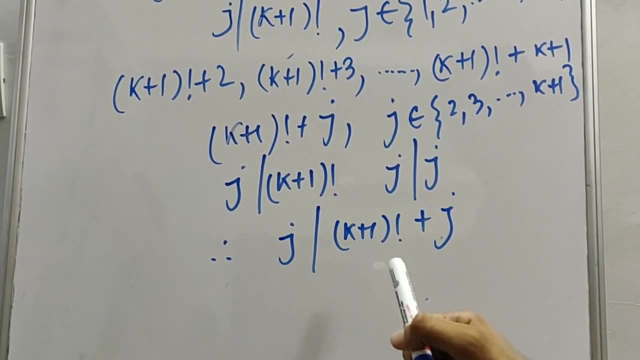 comma till k plus 1.. Now we have already shown that j divides k plus 1 factorial and for any integer j, obviously j divides j. Therefore we can say that j will divide the sum of these two, that is, k plus 1 factorial plus j. So we have shown that j is a factor of the term k plus 1. 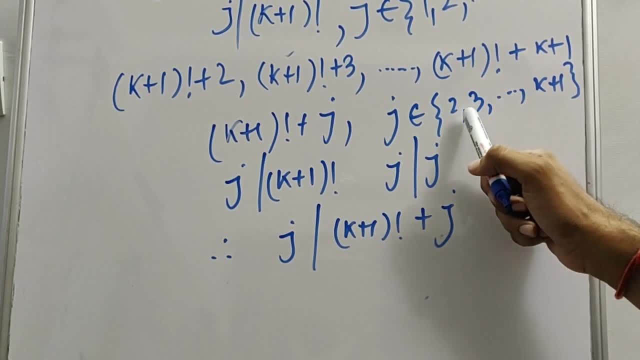 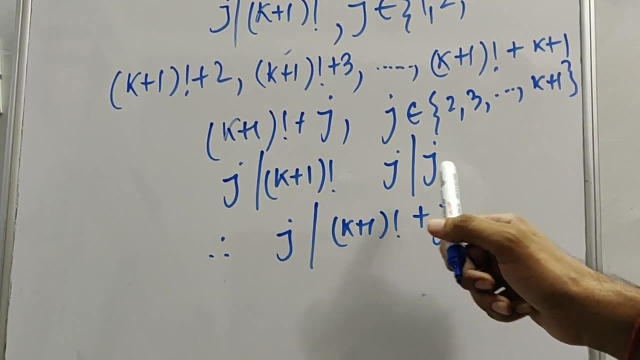 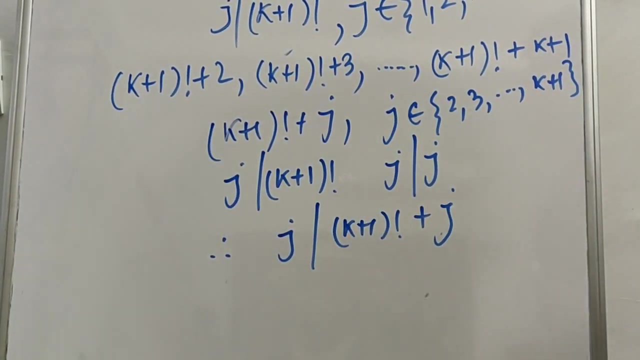 factorial plus j whenever j belongs to the set 2 comma, 3 comma, dot, dot, dot till k plus 1.. Therefore, what we have shown? We have shown that each of the term has an factor. Therefore they cannot be prime. So we have. 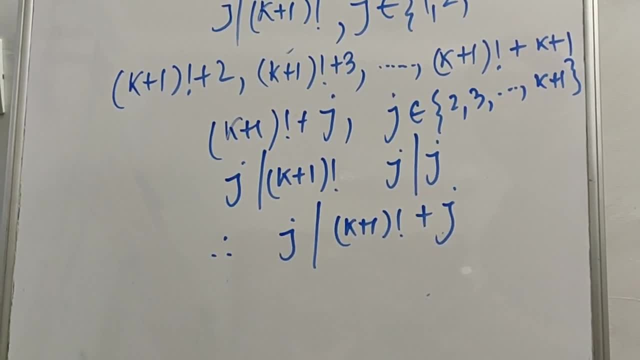 obtained a sequence of k consecutive integers, So this concludes the problem.